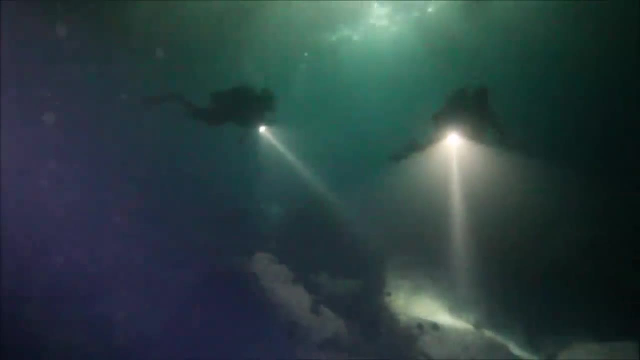 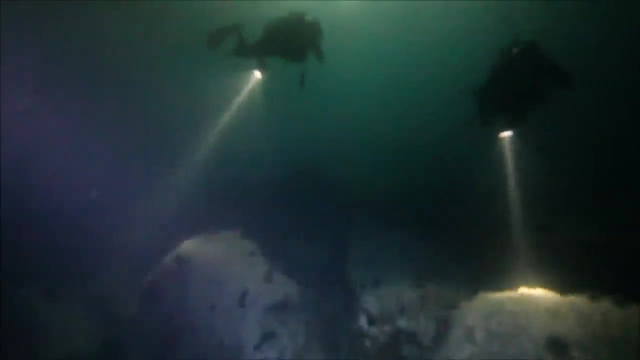 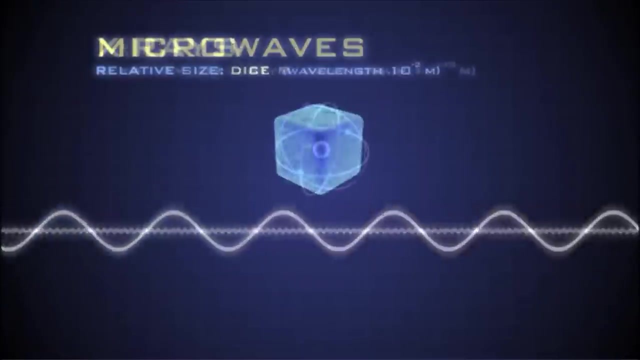 radiation. When we talk about light, we usually mean visible light, which is the light that we can see with our eyes, But there are more types of electromagnetic radiation that are invisible to us, including radio waves, microwaves, x-rays and gamma rays. 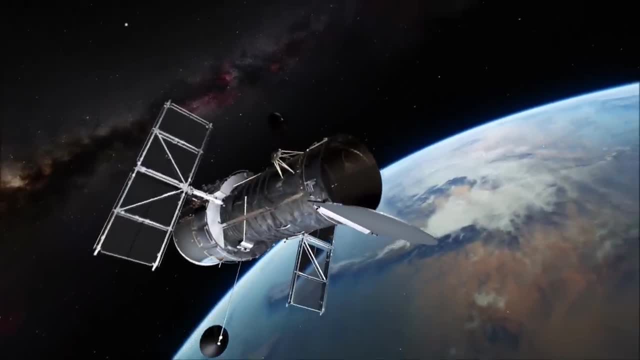 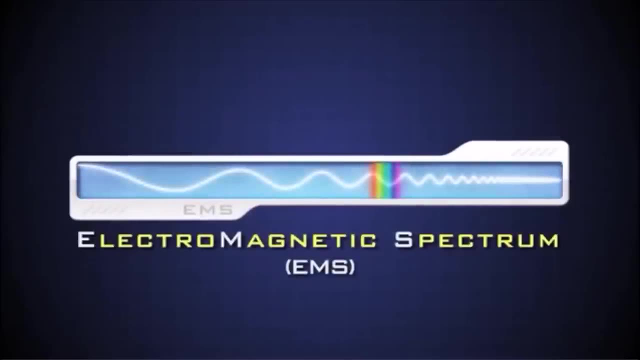 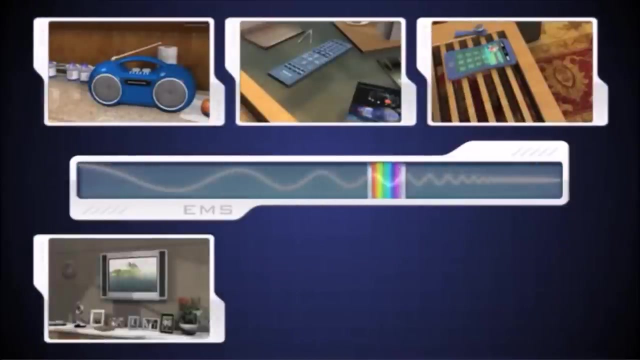 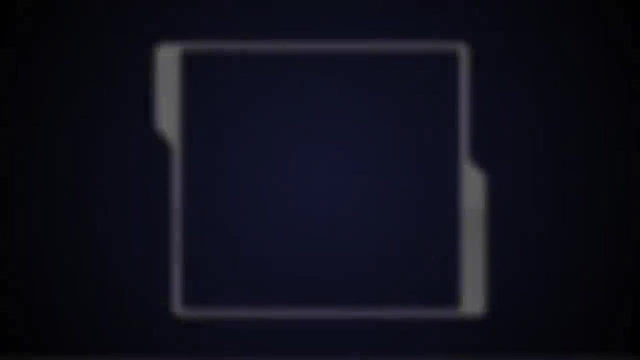 Scientists can detect and measure invisible radiation with special tools. Together with visible light, all these types of radiation are called the electromagnetic spectrum. All electromagnetic radiation travels in waves, but different types have different wavelengths. The wavelength of electromagnetic radiation or light, is connected to how much energy. 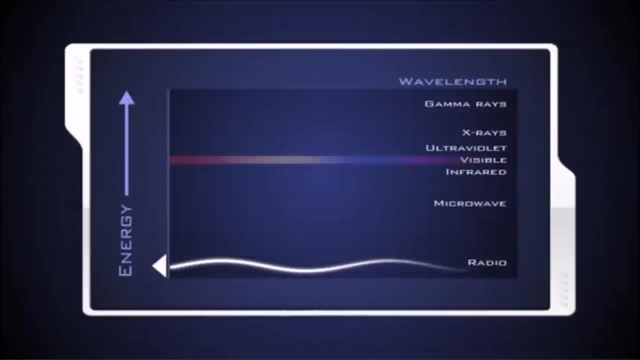 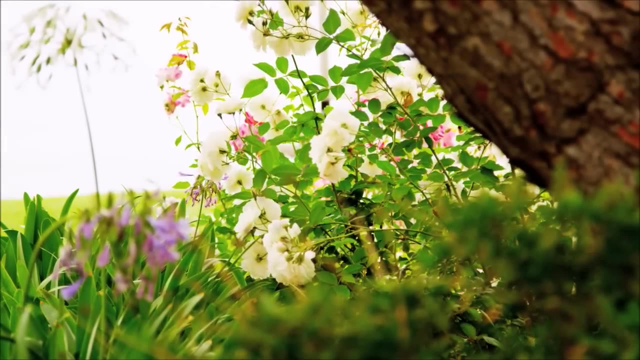 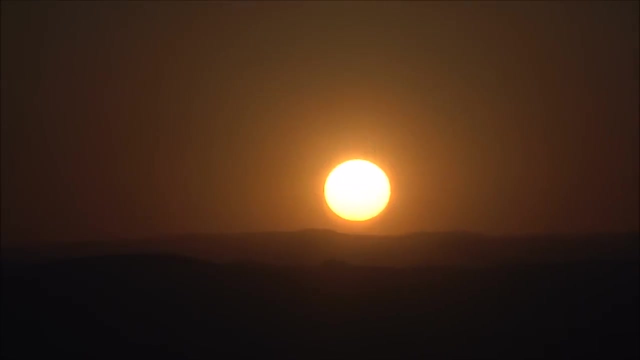 it has. Light with a longer wavelength, like radio waves, has less energy, while light with a shorter wavelength, like gamma rays, has more energy. Visible light makes up only a tiny part of the electromagnetic spectrum, but it includes every color we can see. The most important source of light here on Earth is the sun. 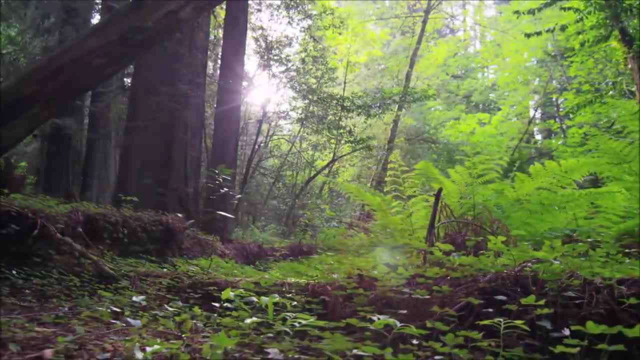 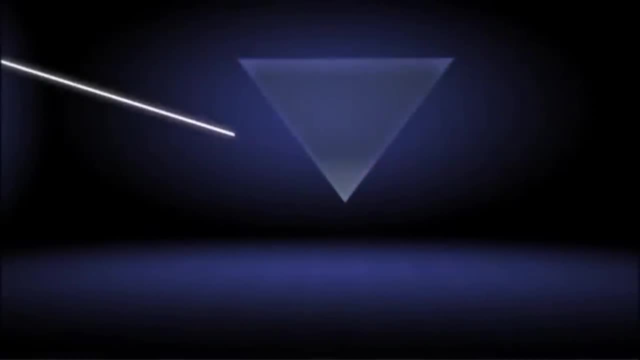 We call ordinary sunlight white light, but it actually includes all light. These colors can be revealed when white light goes through a prism. When light passes through a prism or something like it, it slows down a little bit and bends Some parts of the light slow more than others, and the light spreads out into the colors. 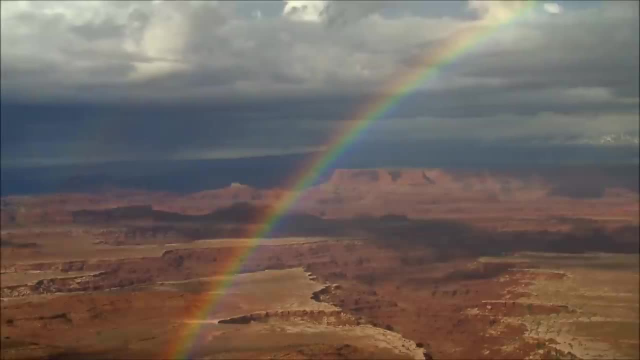 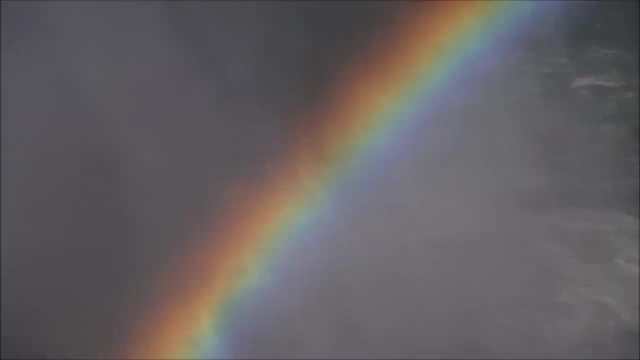 of the spectrum. If you want to see all of the colors in the visible light spectrum, look no further than a rainbow. Rainbows are made when water droplets in the air bend slowly- Sunlight much like a prism. Usually when we talk about a rainbow, we say it is made of seven colors. 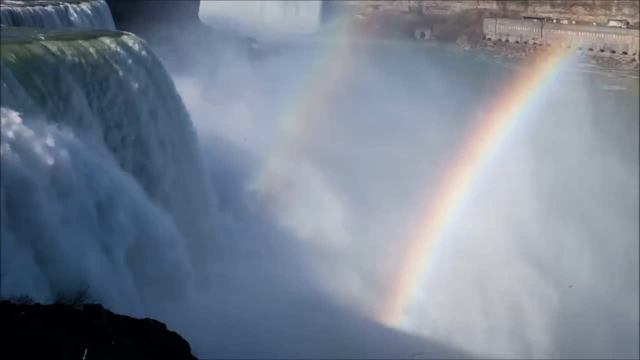 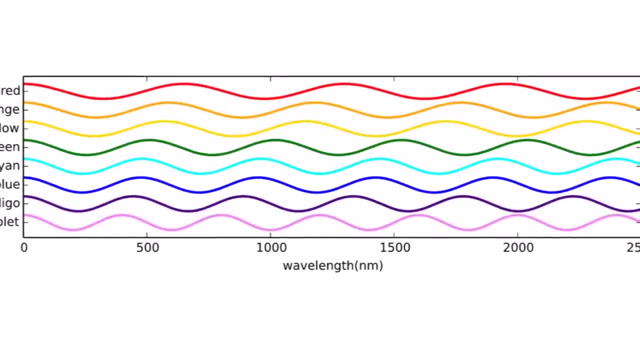 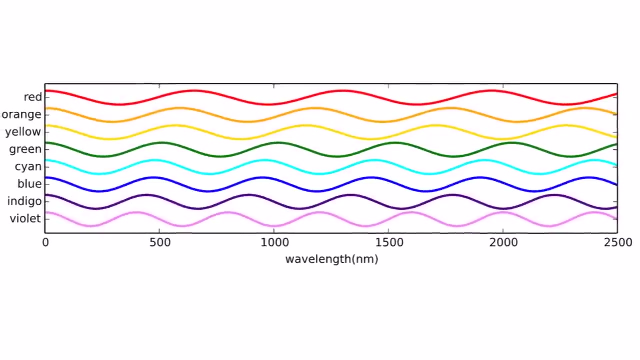 Red, orange, yellow, green, blue, indigo and violet. Each color has a different wavelength. Red has the longest wavelength in the spectrum of visible light and violet has the shortest wavelength. All the other colors have wavelengths in between the two. 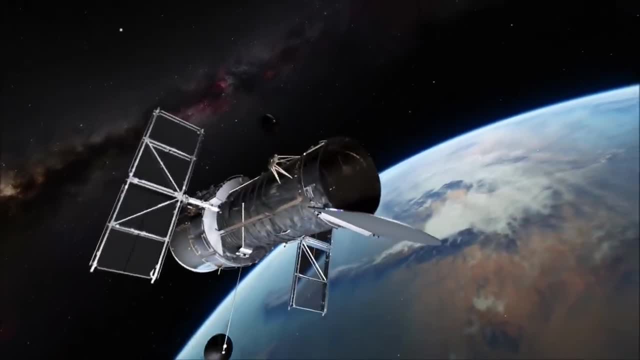 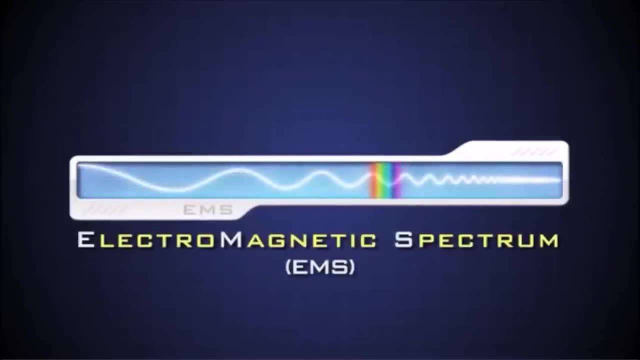 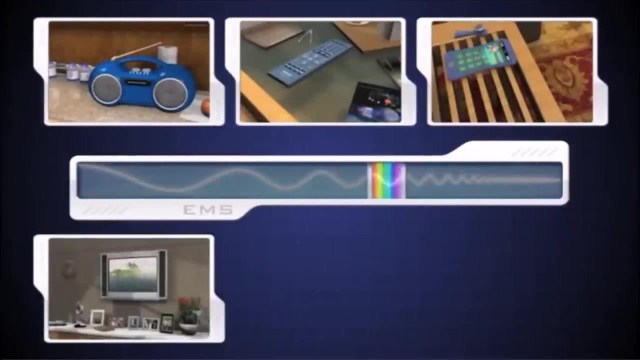 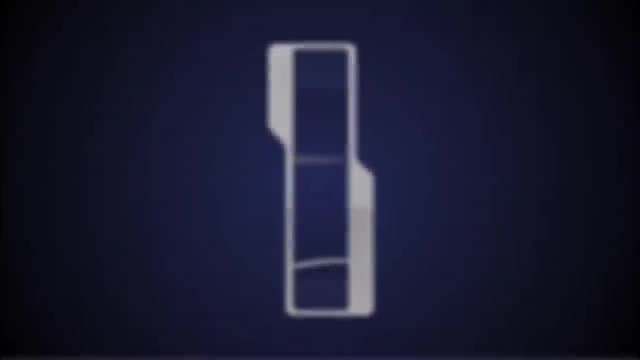 Scientists can detect and measure invisible radiation with special tools. Together with visible light, all these types of radiation are called the electromagnetic spectrum. All electromagnetic radiation travels in waves, but different types have different wavelengths. The wavelength of electromagnetic radiation or light, is connected to how much energy. 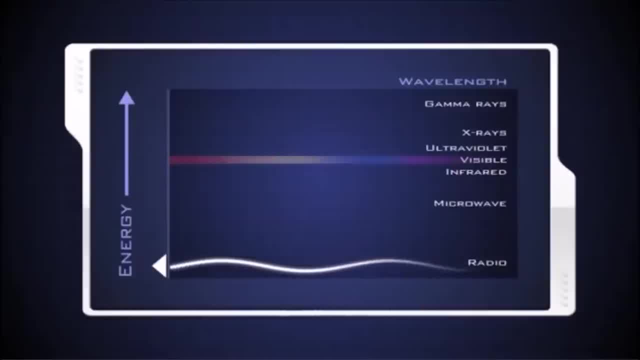 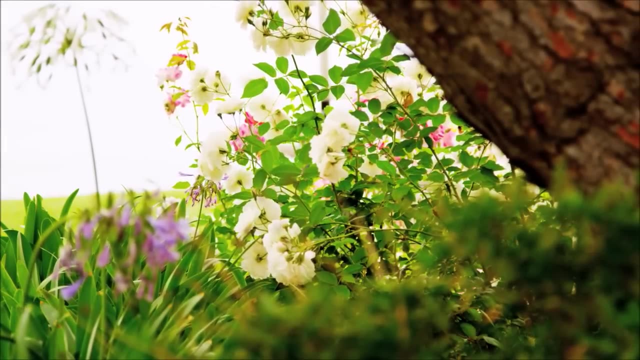 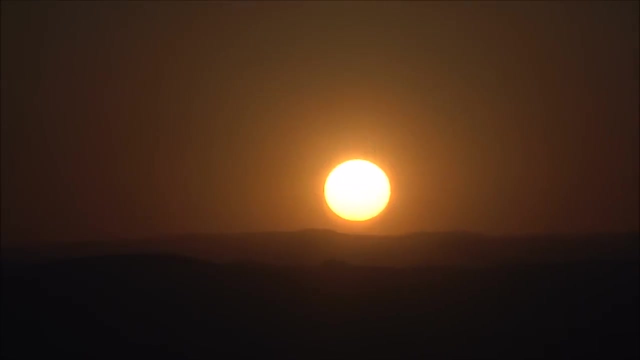 it has. Light with a longer wavelength, like radio waves, has less energy, while light with a shorter wavelength, like gamma rays, has more energy. Visible light makes up only a tiny part of the electromagnetic spectrum, but it includes every color we can see. The most important source of light here on Earth is the sun. 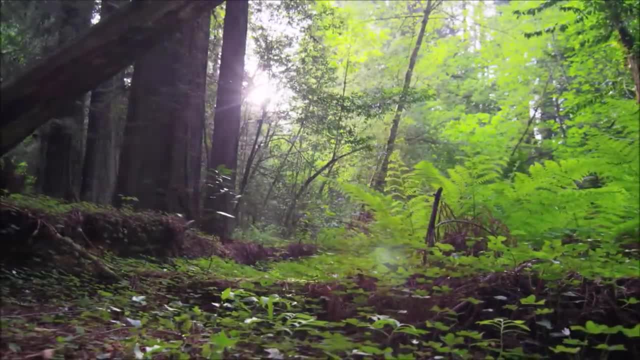 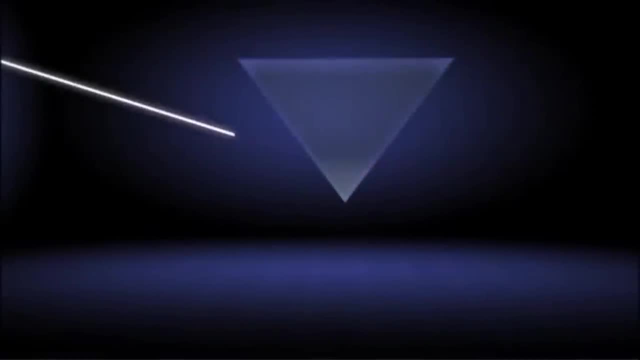 We call ordinary sunlight white light, but it actually includes all the light we can see, All the colors of visible light. These colors can be revealed when white light goes through a prism. When light passes through a prism or something like it, it slows down a little bit and bends. 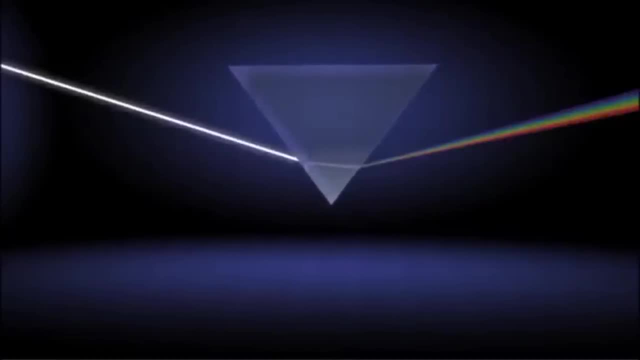 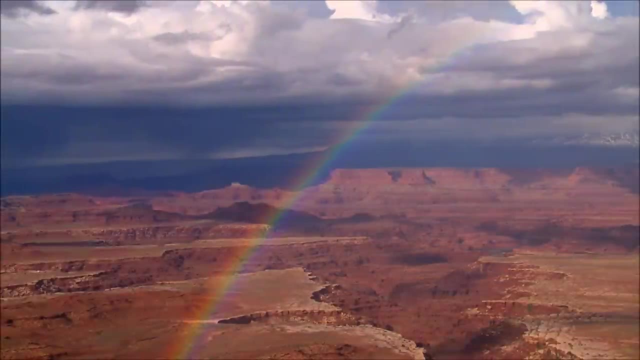 Some parts of the light slow more than others, and the light spreads out into the colors of the spectrum. If you want to see all of the colors in the visible light spectrum, look no further than a rainbow. Rainbows are made when water droplets in the air bend sunlight much faster than light does. 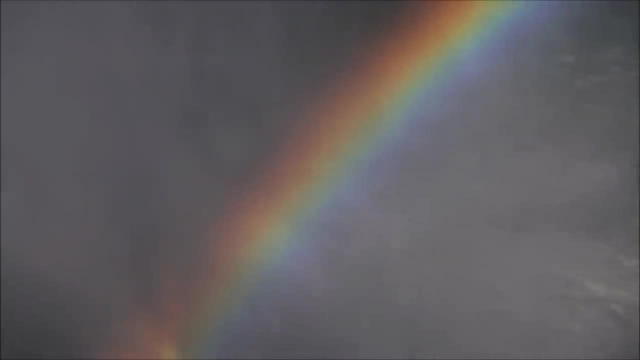 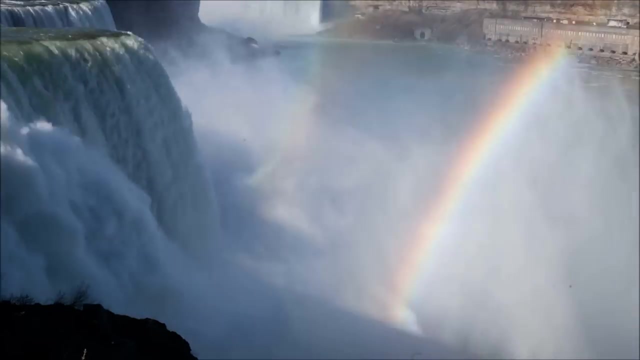 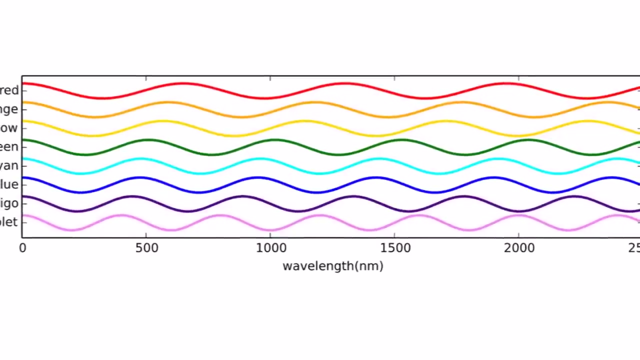 much like a prism. Usually when we talk about a rainbow, we say it is made of seven colors: Red, orange, yellow, green, blue, indigo and violet. Each color has a different wavelength: Red has the longest wavelength in the spectrum of visible light and violet has the shortest. 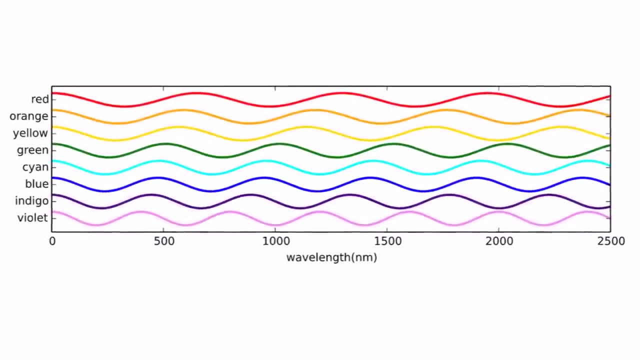 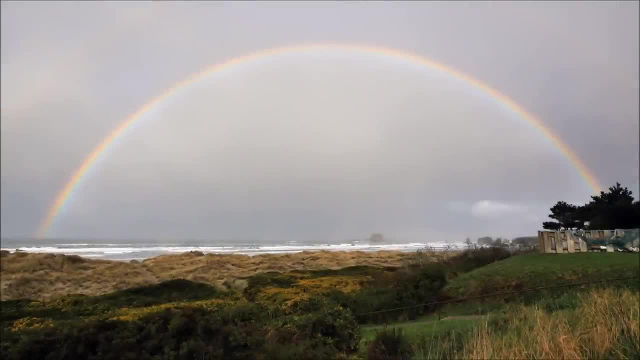 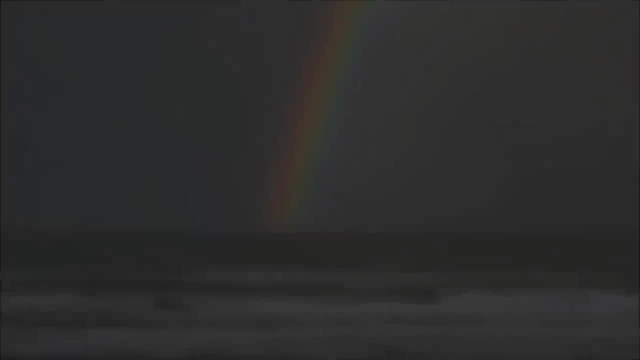 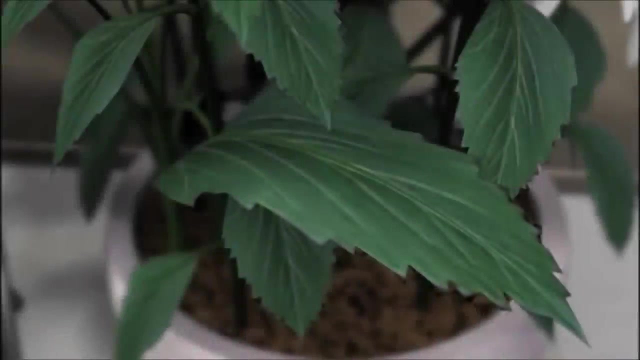 wavelength. All the other colors have wavelengths in between the two. The colors of a rainbow are always in the same order because the colors are arranged according to their wavelengths. Red is always on the outside because red has the longest wavelength, And violet is always on the inside because violet has the shortest wavelength. 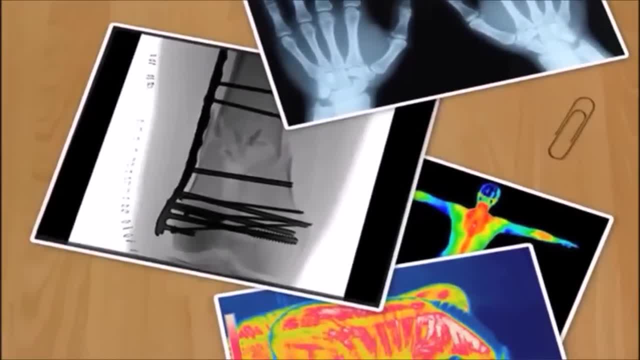 Electromagnetic radiation with a wavelength outside the visible light spectrum is invisible to our eyes. Light with a longer wavelength than the reddest red our eyes can see is called a prism. Red has the longest wavelength. The reddest red our eyes can see is called a prism.